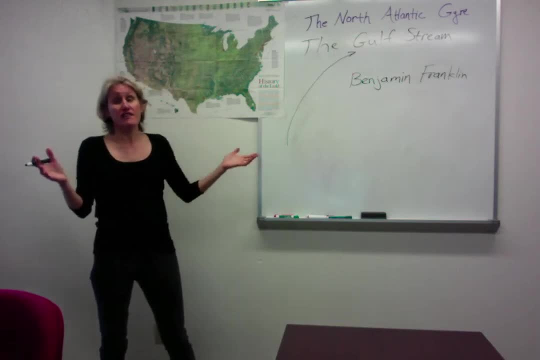 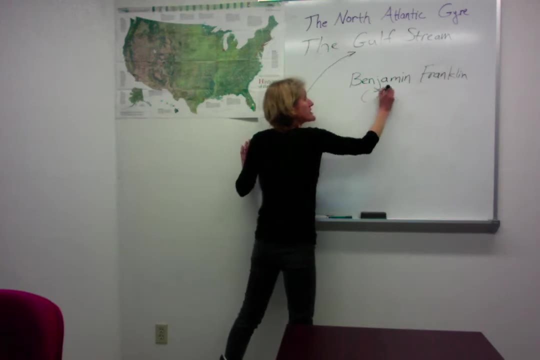 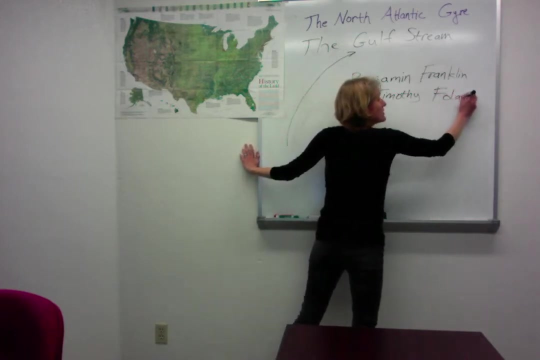 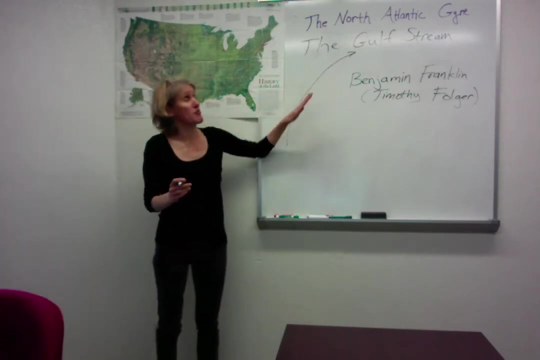 ships were taking longer to get to the eastern seaboard than others. from London was talking to his cousin, the whaler Timothy Folger, who was telling him about this very strong current that they would use to help them chase the whales. Now, Benjamin Franklin. 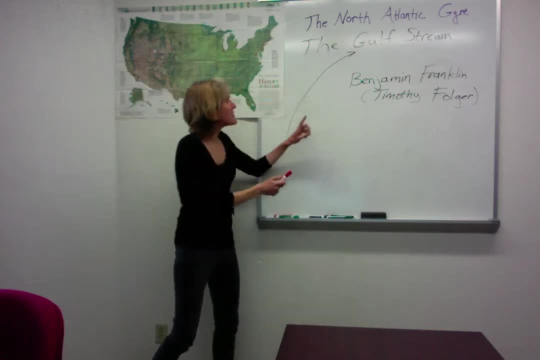 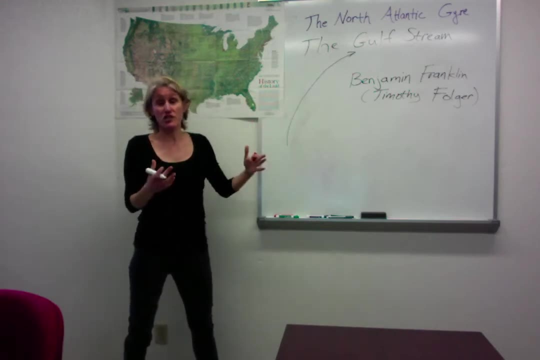 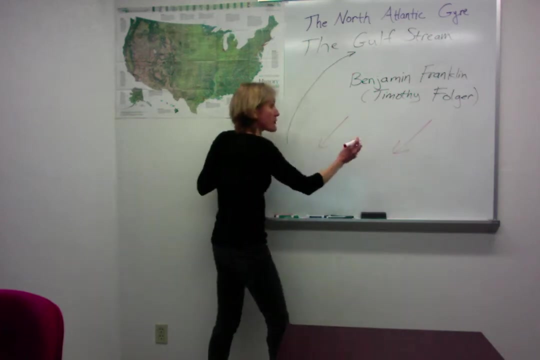 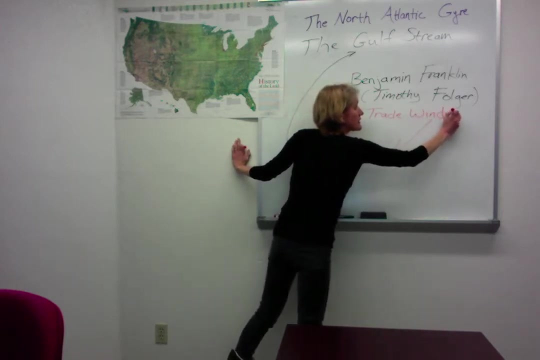 who was the head of the Gulf of Mexico, thought about this, and he thought that the source of the Gulf Stream was most likely due to the fact that there were very strong perpetual winds- the trade winds- that were always blowing from east to west. 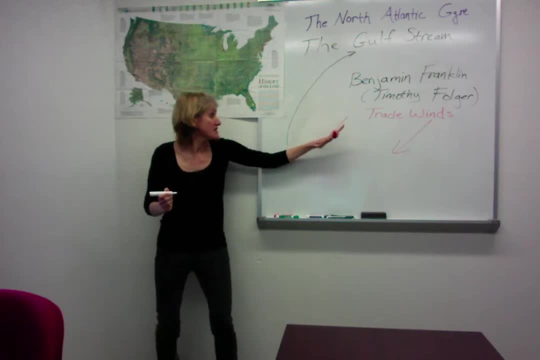 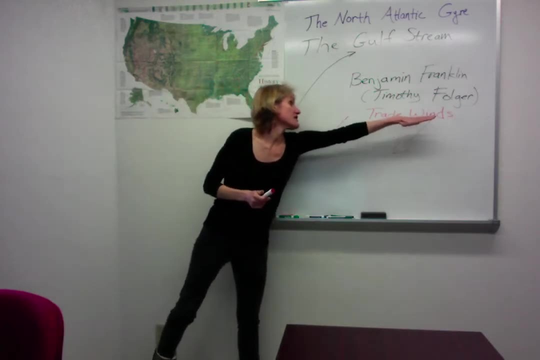 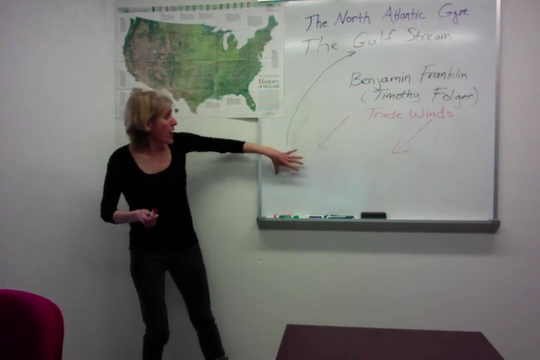 to west, in a in a um south westerly direction, and these trade winds were used by sailors when they were coming across from europe to the americas. he believed that the trade winds were actually piling up waters down along the coast of south america and that because the water got piled up, 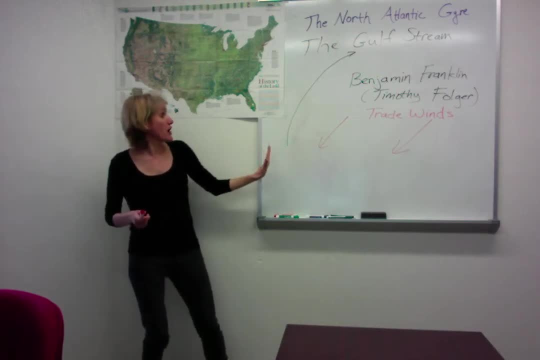 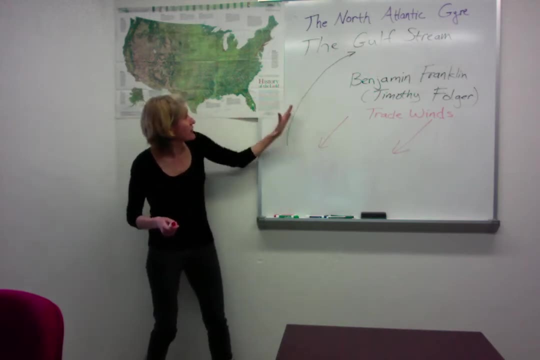 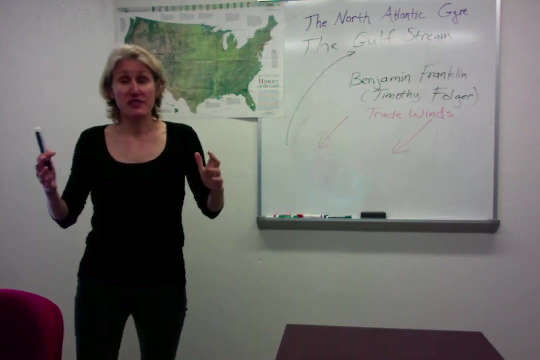 there was a higher pressure gradient here, and so the waters then would move upward into the gulf of mexico and then through the straits of florida and formed the gulf stream. another explorer who put who did a lot of work on the gulf stream, was james rennell. 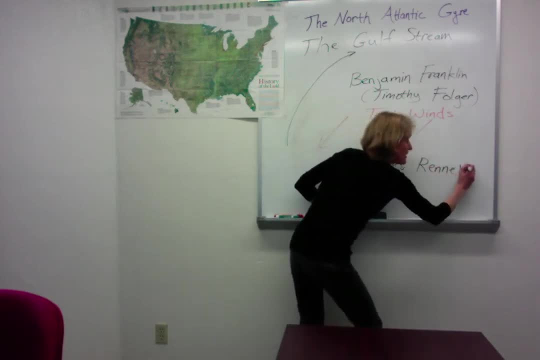 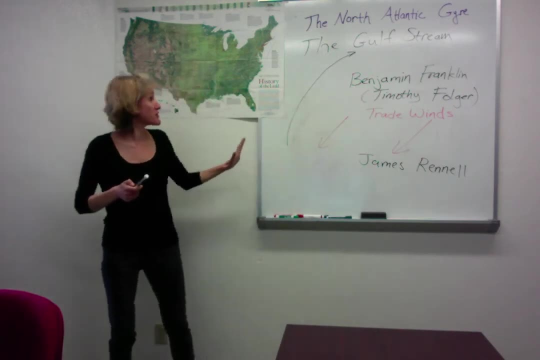 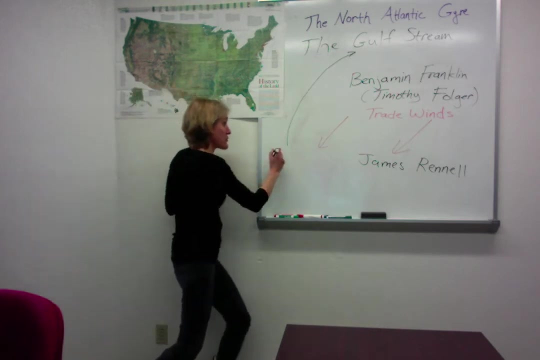 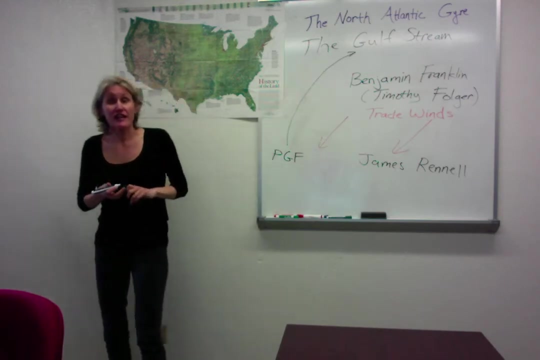 james rennell agreed with benjamin franklin that the trade winds were in fact the source of the gulf stream and that it was due to the winds piling up the water and creating this high pressure gradient force that then would push the waters in this direction. he called this a stream, current now. 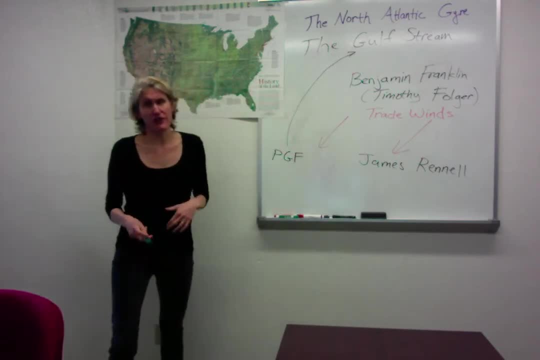 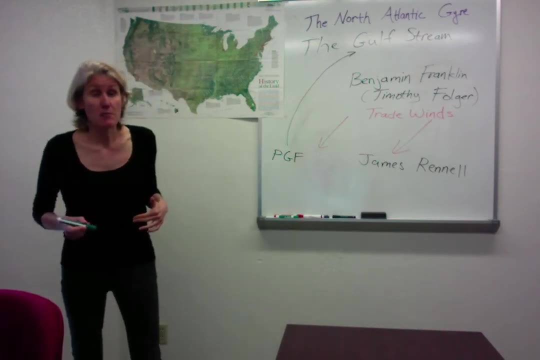 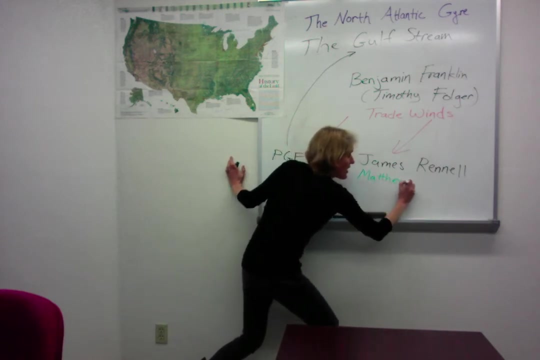 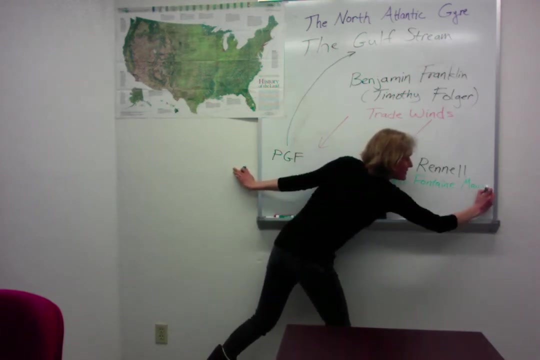 another person who did a lot of work in oceanography and has really helped to develop many oceanographic charts that we use today. um was maury matthew, fontaine, maury, and maury did not agree with rennell and franklin. he thought that there's no way that the wind was going to be in the gulf stream. 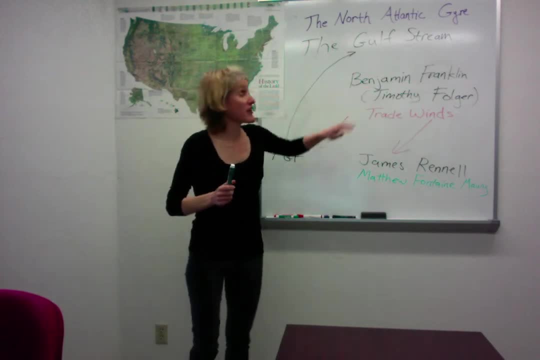 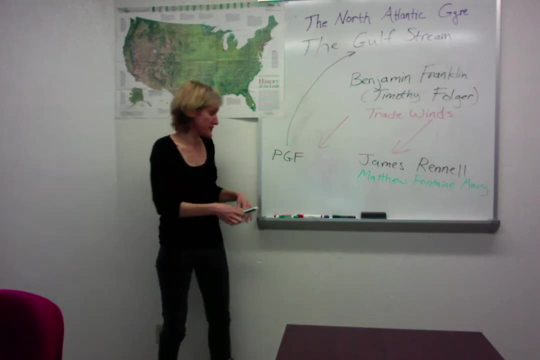 and maury did not agree with rennell and franklin. he thought that there's no way that the wind was going to be in the gulf stream, no way that the winds were strong enough to be the only reason that we had the gulf stream. and his reasoning was this: well, if here in the 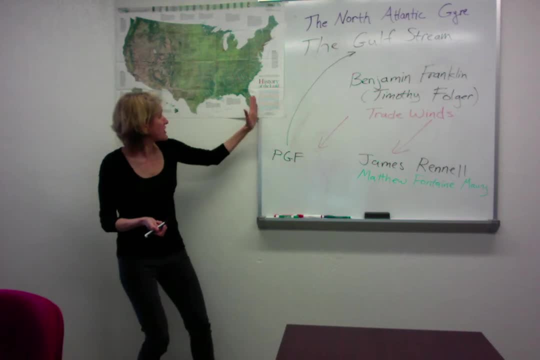 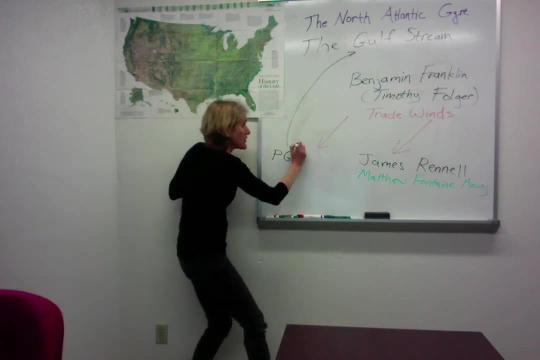 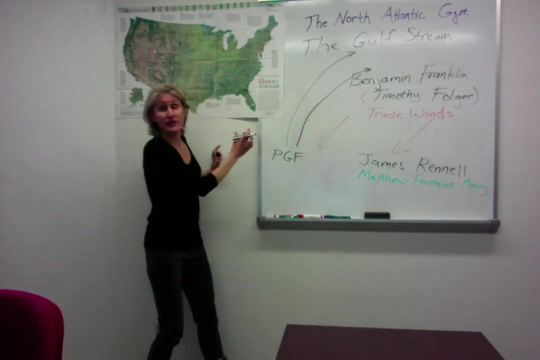 straits of florida. the same volume is transported through the straits of florida. that then passes by cape hatteras, and he knew that the gulf stream was narrower in the straits of florida and it became wider in cape hatteras. therefore, he reasoned, cape hatteras must have a shallower sea floor. 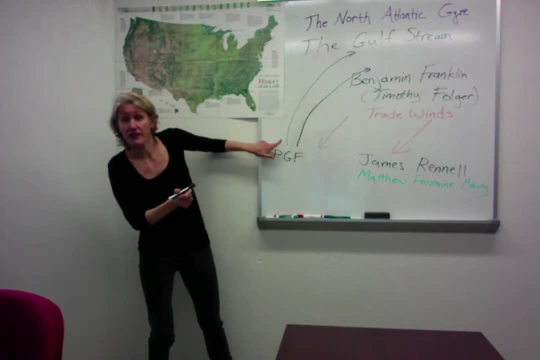 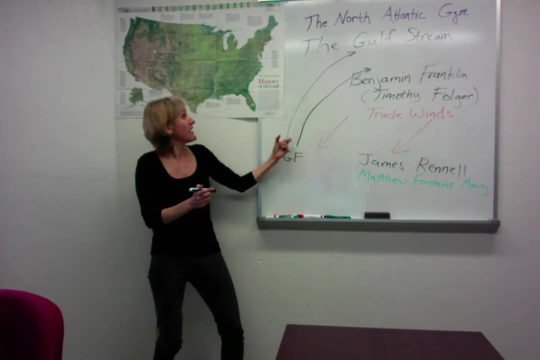 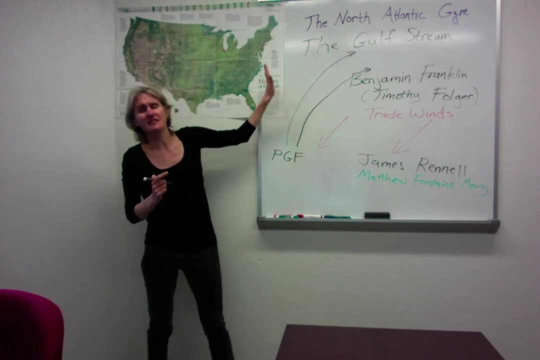 than the, than the sea floor is in the straits of florida. so that means that the water is that the sea floor is deeper in the straits of florida than it is in at cape hatteras and therefore in his mind, the water had to go uphill because he was thinking about the sea floor and 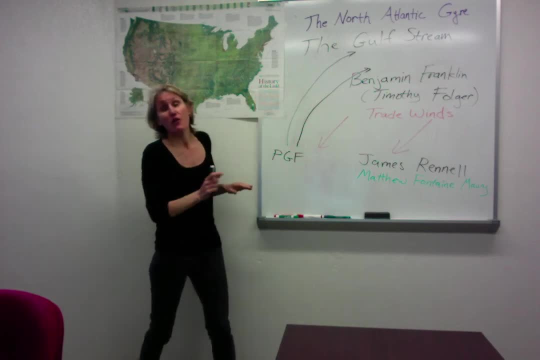 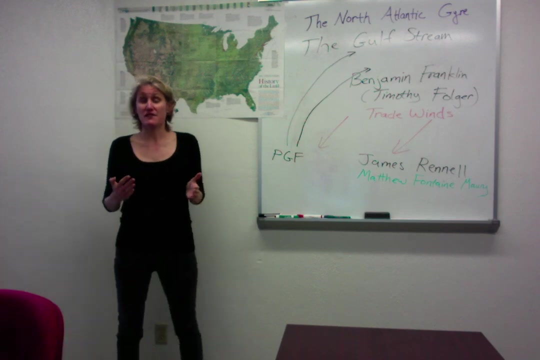 the fact that the water had to go up the sea floor. we know that this is not true, because we have studied the fact that that it is a pressure gradient force that is determined not by the sea floor but, in fact, by the sea surface height or, even more specifically, by the isopictals. 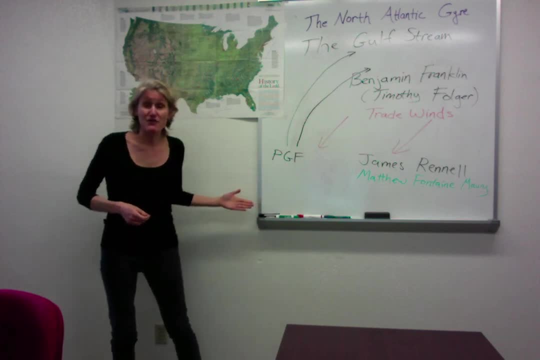 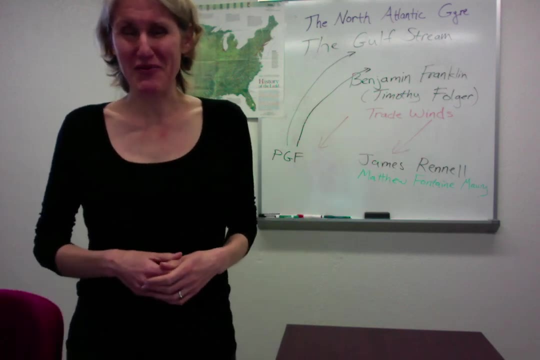 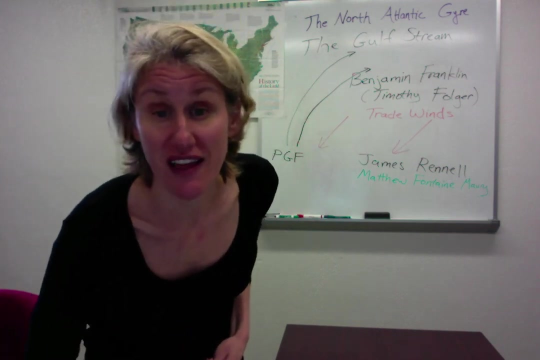 and that's what gives us our pressure gradient force and allows us to have the gulf stream all right. the next video i want you to watch is a much nicer video on youtube, looking specifically at benjamin franklin's discovery of the gulf stream and the chart that he drew, which is still accurate today.